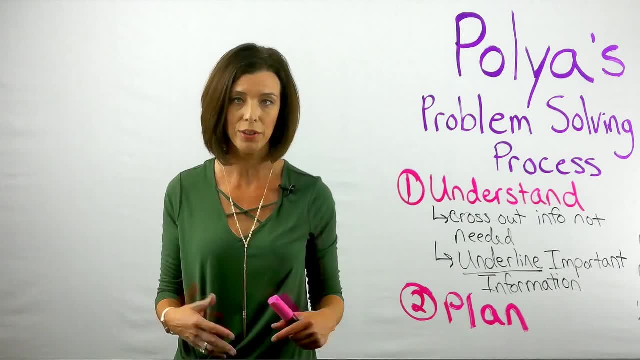 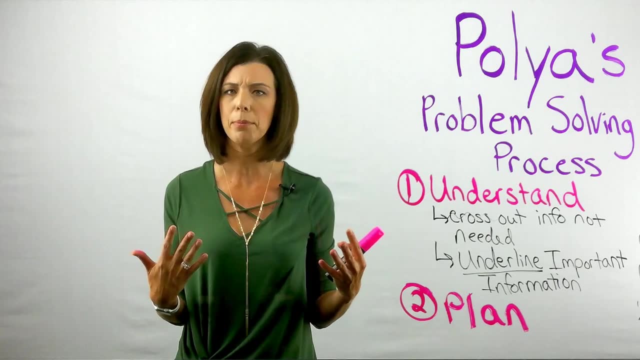 Your strategies for problem solving might include making a drawing of your situation, Maybe coming up with an equation, looking for a formula working backwards. all of these are great problem solving strategies. There's many more. I want you to be recording these in your nu. 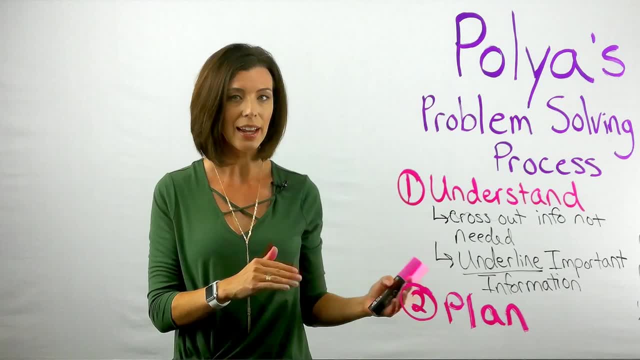 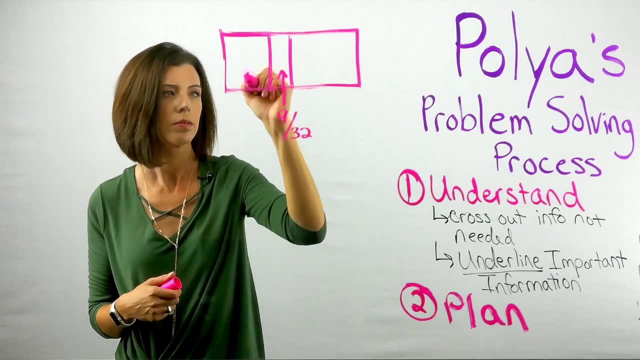 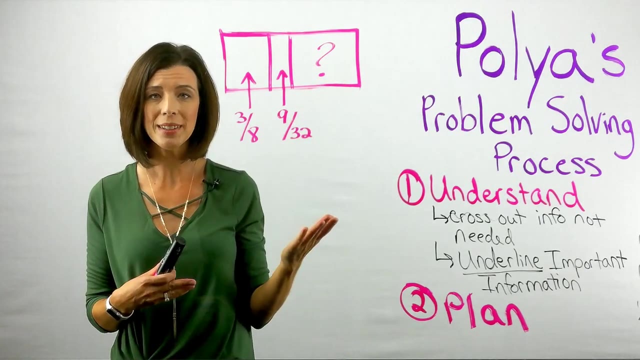 these in your notebook. so we're going to make a plan for our problem. I'm going to go ahead and draw our picture. once I've got this drawn, I can see that I need to solve for this piece right here, and it just so happens that that's the portion. 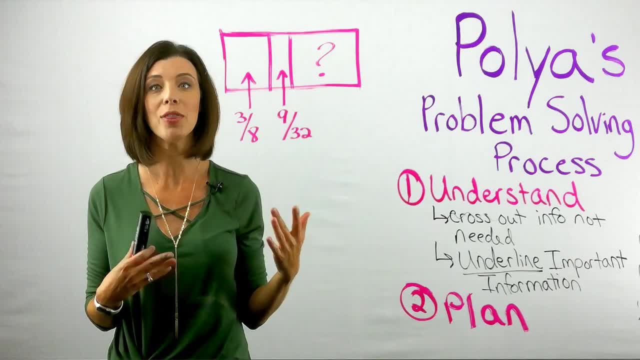 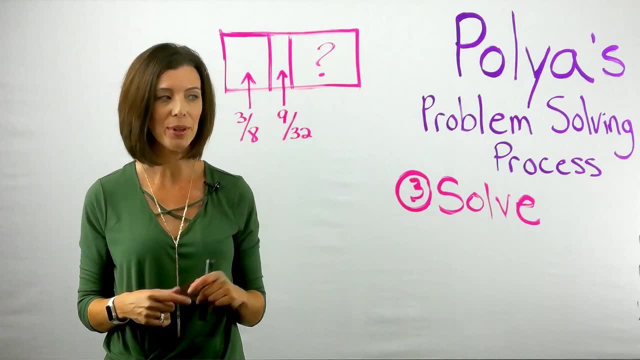 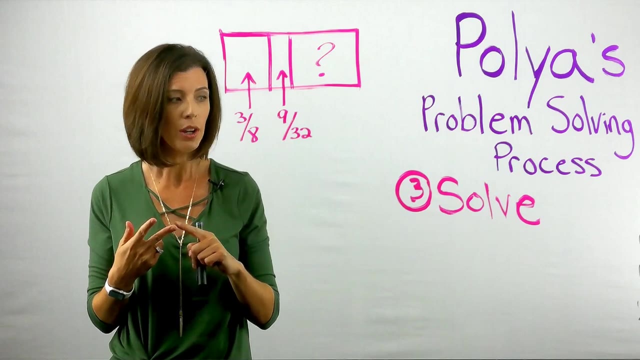 of students that voted for the zoo. again, I'm not getting hung up on the zoo because it doesn't really matter in this case. okay, so now we're ready for step three, which is where we solve. we've already crossed out our information that we didn't need. we've underlined our important information. we've understood. 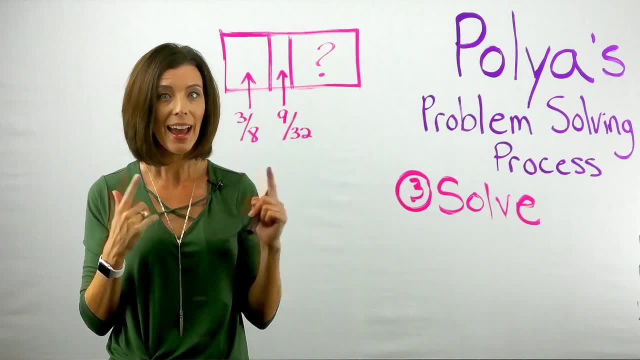 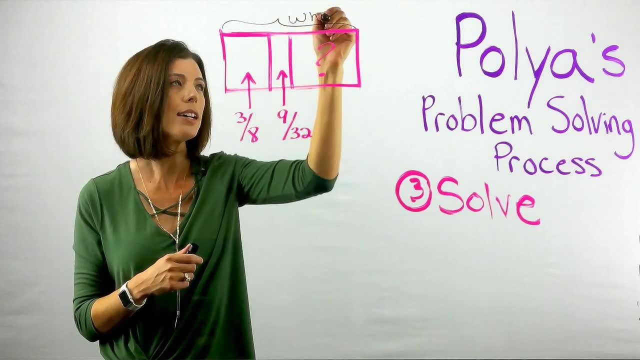 the problem. we've made a plan of how we're going to get the solution, and now we're ready to solve. so I know that my whole here- this is my whole class in this case- can be represented by a one. so I have two options here, and this is: 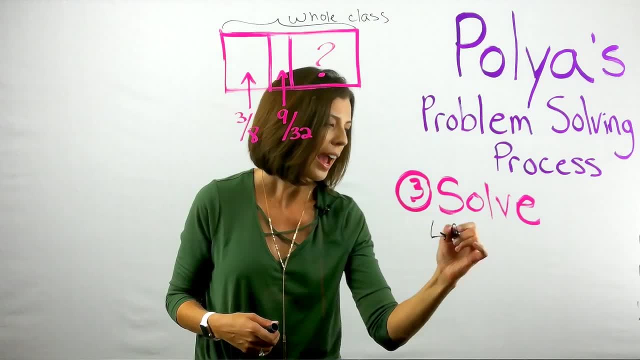 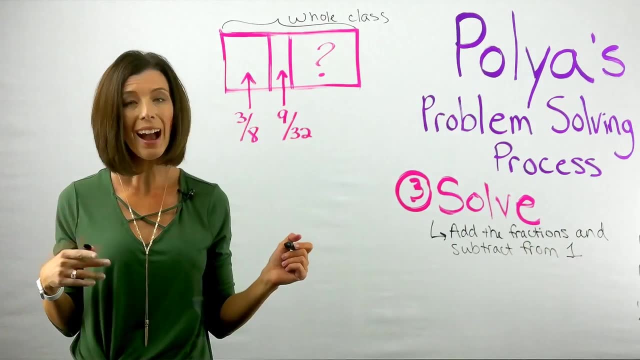 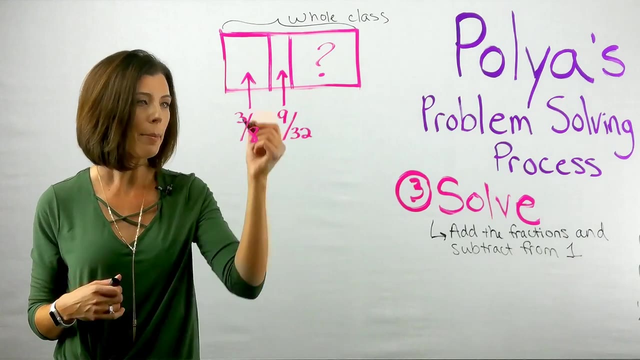 where I'm thinking about my options to solve. I could add the fractions from first and subtract from one, or I could start with the whole class and subtract each part. I'm going to go ahead and do the first one. so I'm going to add three eighths and nine thirty seconds, and I know that I need to get common. 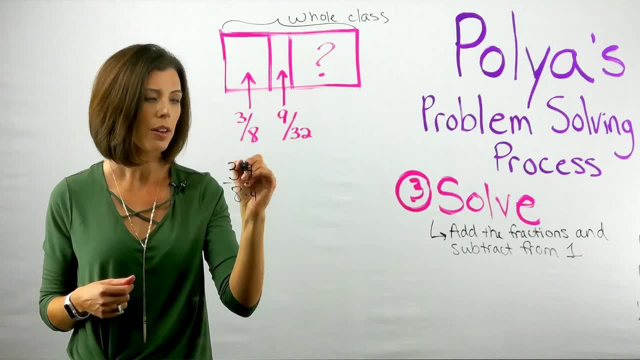 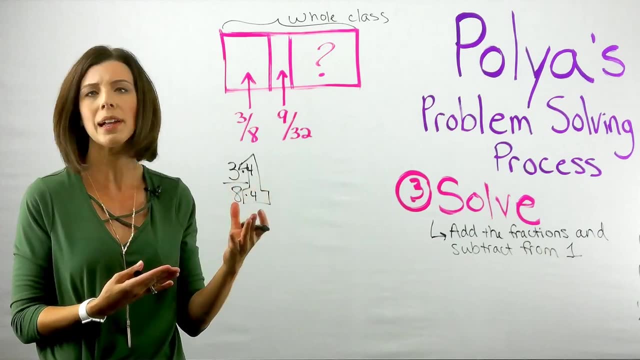 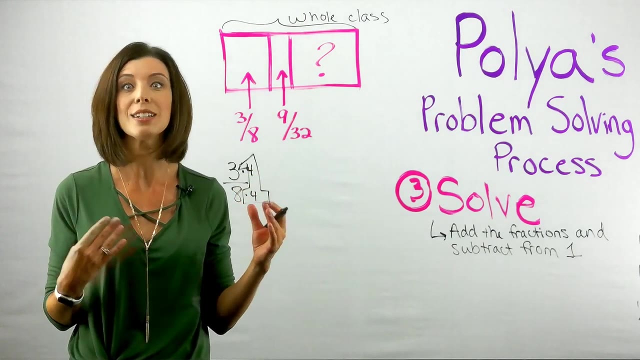 denominators. and right here let me point out as well: we know that I'm allowed to multiply. sometimes students are confused like: why am I multiplying this fraction by four before? why is that allowed? because we're really just multiplying by one, so we're just cutting the pieces into smaller pieces. so now I know I have 12, 30 seconds and I'm going. 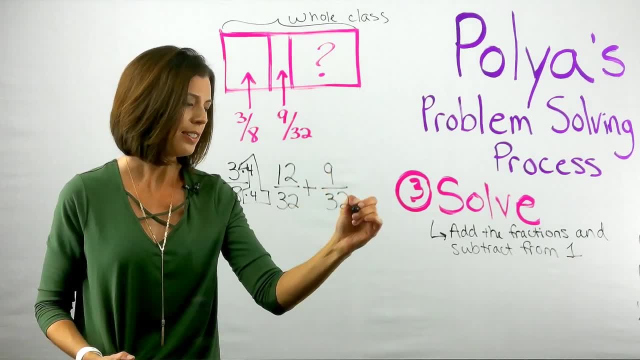 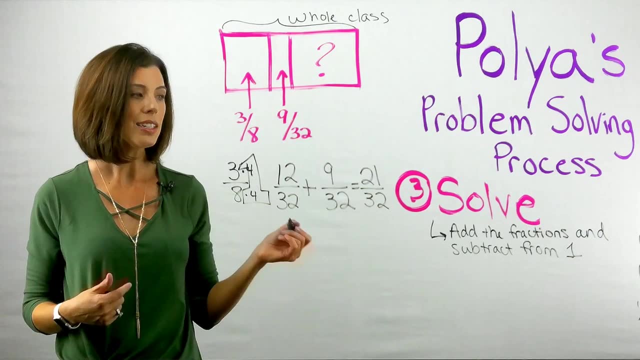 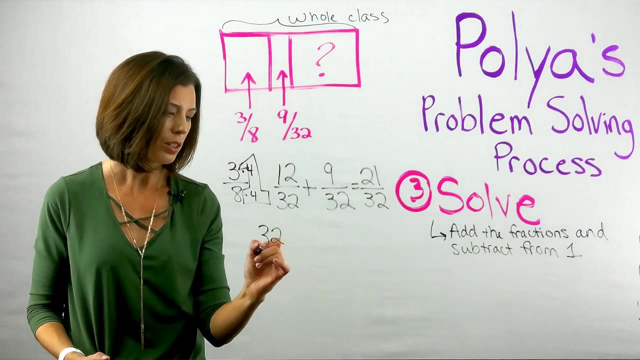 to add that to my 9 30 seconds, which is going to give me 21 30 seconds. now I can go ahead and subtract this from my whole, so I know that my whole is one whole, but if I'm dealing in 30 seconds, I want it to be 32.